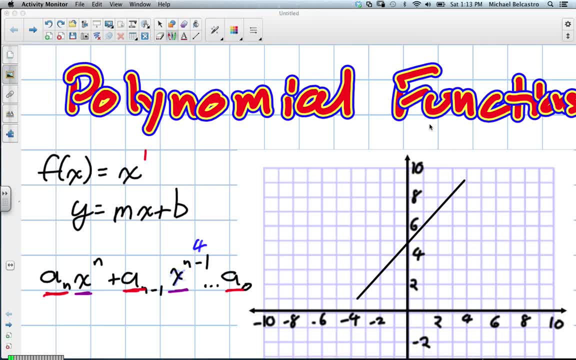 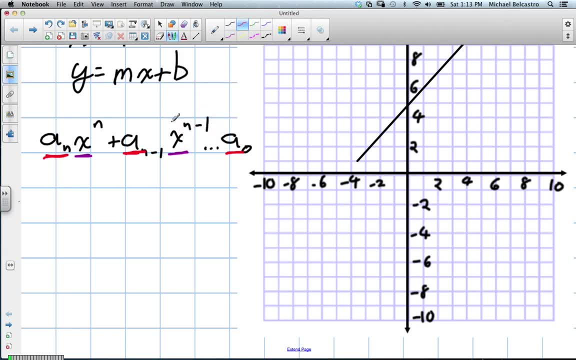 So what we're going to do is actually go about putting these in order using a linear function. So our linear function, like we said, can kind of be written like this: They have a x and it's to the power of one. 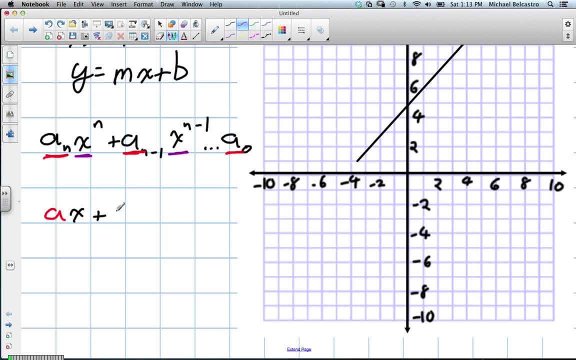 And then you would just say plus, and they usually put a naught, A naught meaning some constant term. So this would be our linear function And technically this would be a1 in this case. The next type of function you would learn about, probably in grade 10, is a quadratic function. 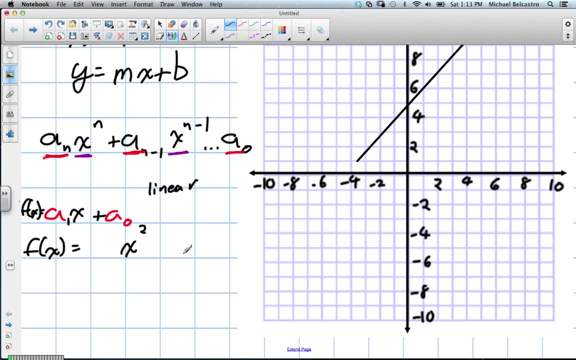 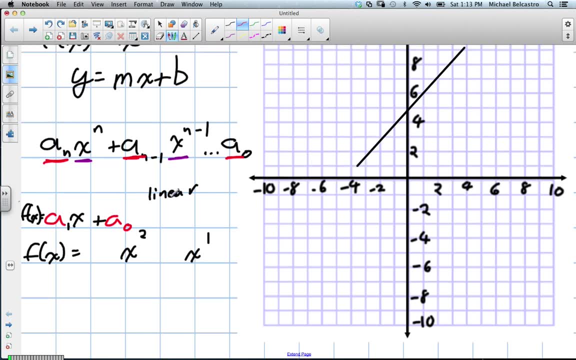 And if you remember that one starts with a squared, Then what we have is an x to the power of one And then finally some constant term. So the same idea here is all they've done is. they said you have a. you could say it's the second coefficient. 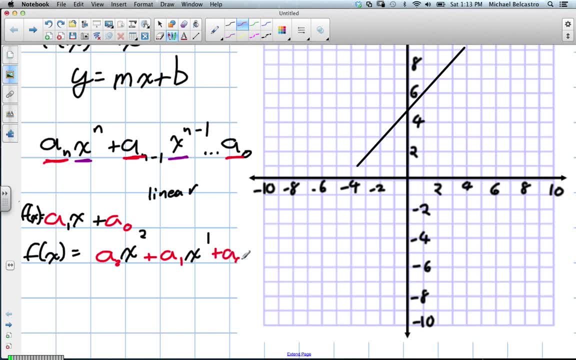 plus a to the first coefficient, plus a naught again being some constant term, And we can continue to go up and up and up with this. So this is a function we're a little more used to. We usually saw it like this: 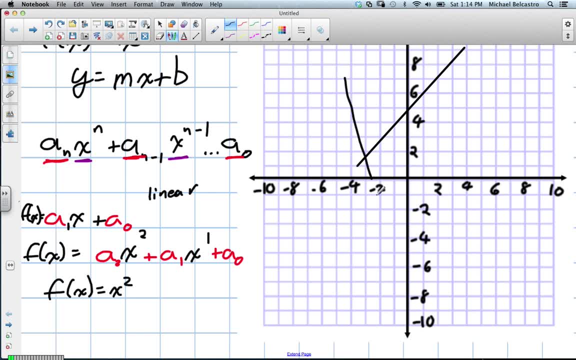 f of x is equal to x squared And we know it represents some parabola, Something like this. That would be our second one there. The first one was a linear, The next one we had is a parabola or a quadratic. 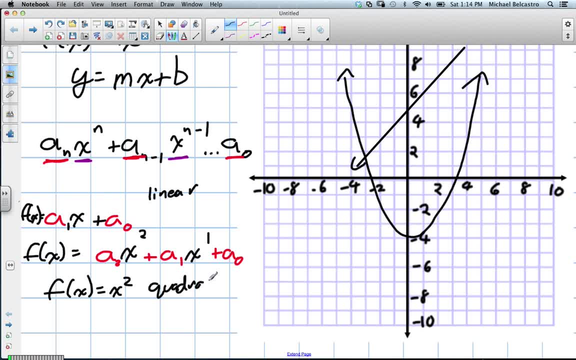 So this is a quadratic function, So this is quadratic. We'll kind of highlight them. for us, Linear was in yellow, here Quadratic functions are the ones we have in green. So these are quadratic functions And again, a just stands for some number. 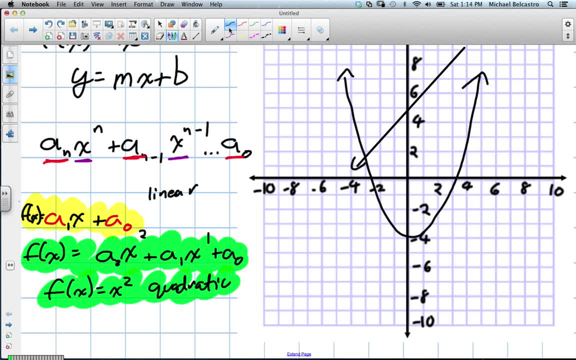 And we can put examples in for this. An example of a linear function could just be: f at x is equal to 3x plus 1.. Okay, So that would be a linear function. For a quadratic function, we could have: f at x equals, let's say, 2x squared plus 3x plus 1.. 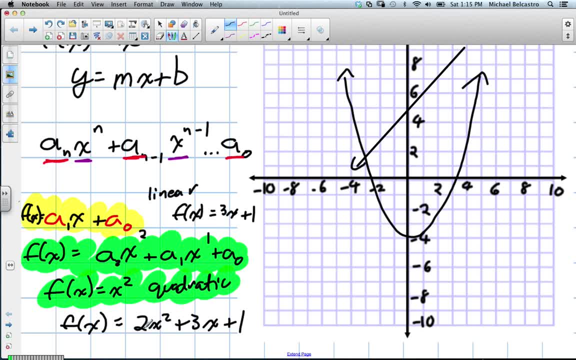 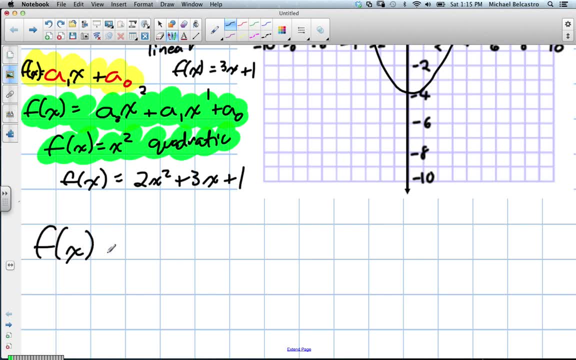 And you know what we'll do. We'll just keep adding on to the original one we had. Okay, So we've just added another variable to it, And what it does is changes the shape of this function. The next one is a cubic function. 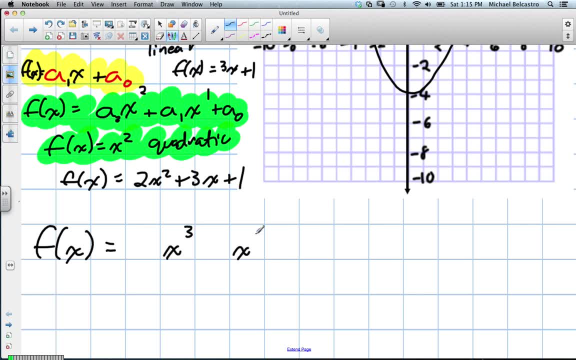 Same idea. The only thing is we start with x to the power of 3., Then we have x to the power of 2., Then we have x to the power of 1. And then a constant term, And they would represent that with: 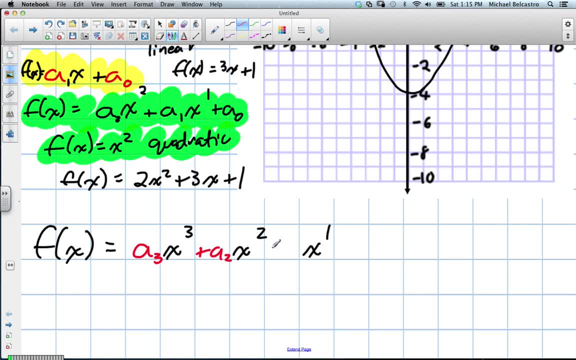 A3 plus A2 plus A1 plus A0.. Okay, You notice how we continuously just keep adding another term to it. Okay, And this is going to give us a completely different shape on a graph- We'll go ahead and check that out in a minute- what it's going to actually look like. 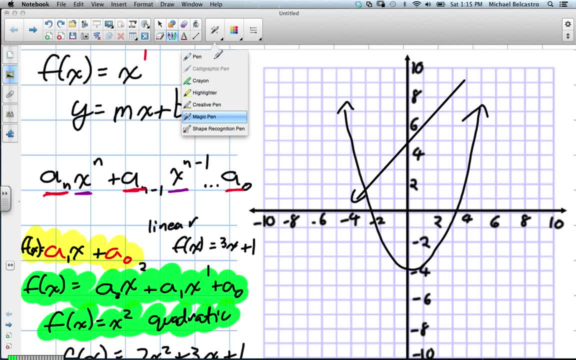 But the general idea to this type of shape is something that actually goes up, comes down and goes up again. Okay, So I'm going to do the new ones in different colors here, So quadratic and linear we're used to seeing, Okay. 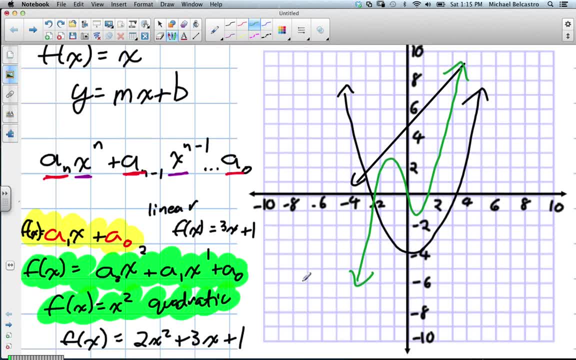 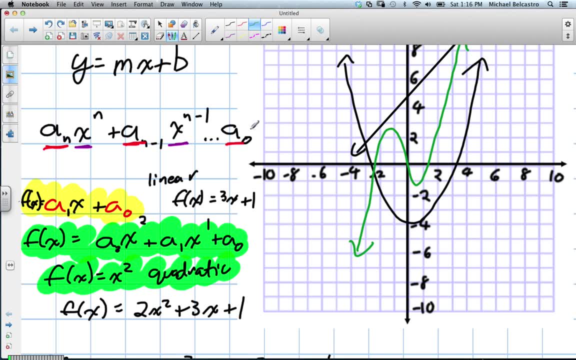 And one way to look at it is the power of the polynomial. essentially, the number of turns in the graph would be kind of 1 less than that, Okay. So what I mean by that is, if you notice well, 1 less than to the power of 1, which is a linear. linear is to the power of 1.. 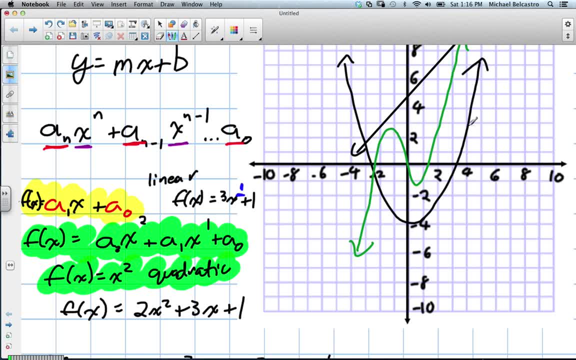 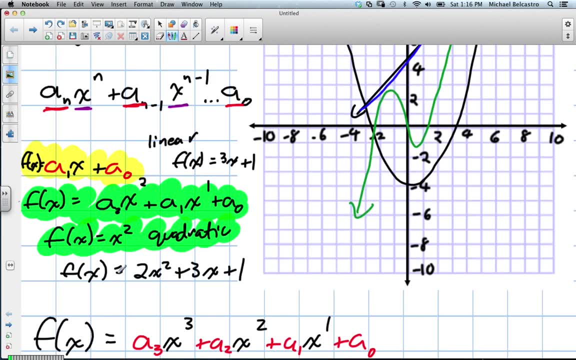 If I go 1 less than that, that means there's no turns in the graph. Okay, 0.. 1 less than 1 is 0. So it's just a straight line In a quadratic function. it's the power of 2.. 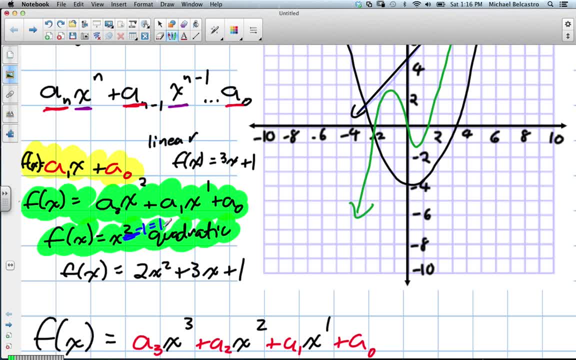 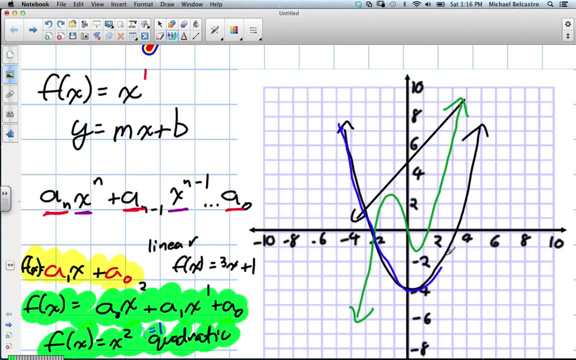 So 1 less than 2 is equal to 1.. So that means there's 1 turn in that function. So let's say we're going from left to right, It goes down and then it turns once. That gives us an idea of a quadratic function. 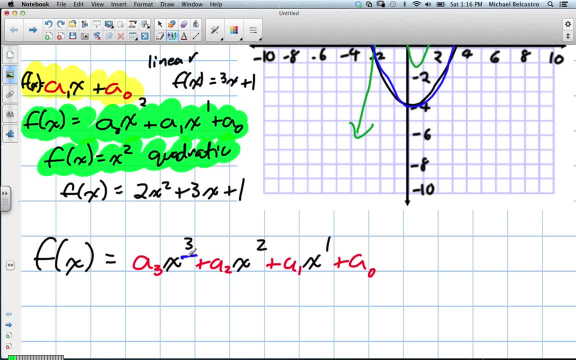 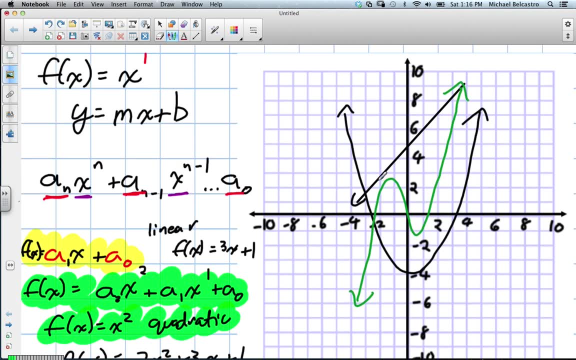 Okay, A cubic function is to the power. the highest power is 3.. So 1 less than 3 gives us 2.. So it's saying it has 2 turns. So again, if we're going from left to right, we go up, we turn directions once and then we turn it again. 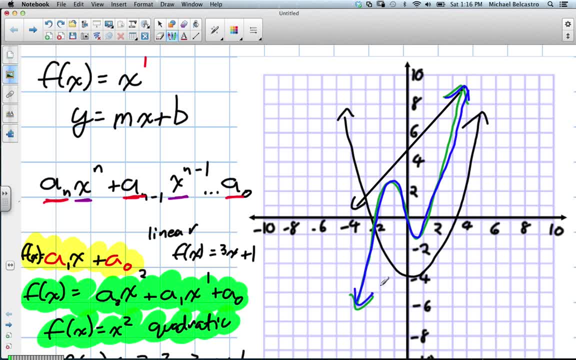 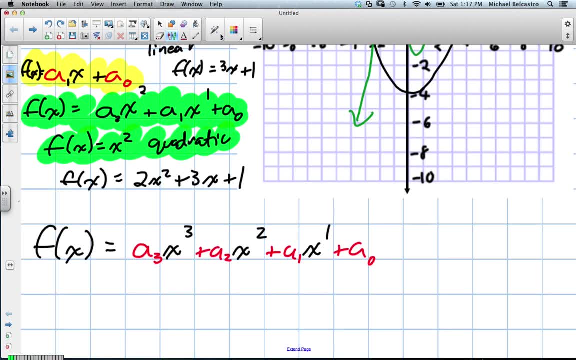 Okay, So that's the idea of a cubic function Essentially. every time we add a term to it, we just essentially add another term to the function. So let's talk about so again. that was cubic. Cubic is a green function here. 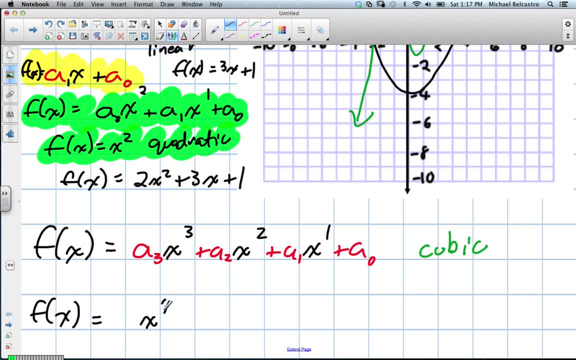 f at x is equal to. now we have x to the power of 4.. 3, I'll just write them in and add the variables after 3,, 2,, 1, and then some constant terms. So we know we're going to have 4 coefficients: a3, or a4, a3, a2, a1, and then probably some constant term. 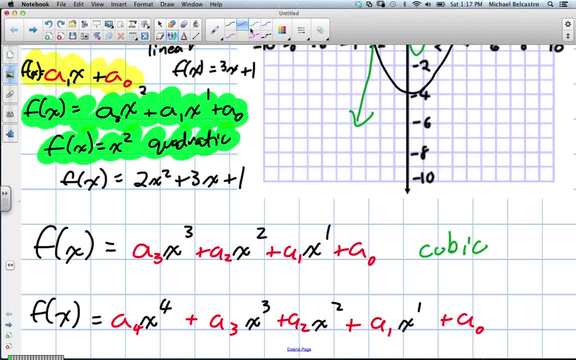 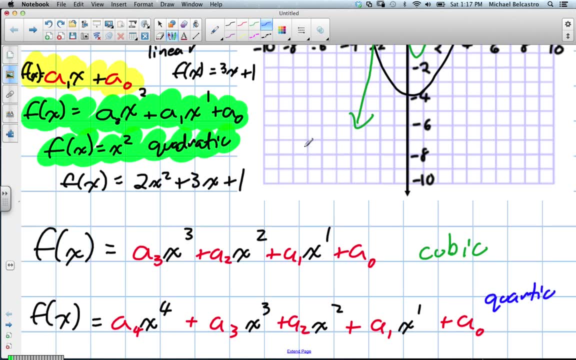 That's what these are, all standard forms, And this is called a quadratic function, Cubic Cortic, sorry, And what we're going to do with that is again because it's to the power of 4, 1 less than 4 is 3.. 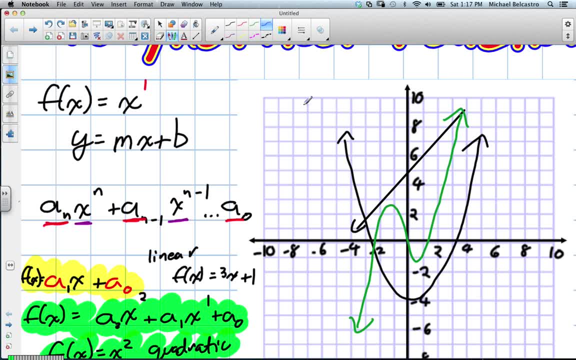 So this one has 3 turns, Okay. So think of it like a function that goes down: 1 turn, 2 turns, 3 turns, So it almost gives us a W shape. Okay, And again, for every one we add to it, we'll do it. 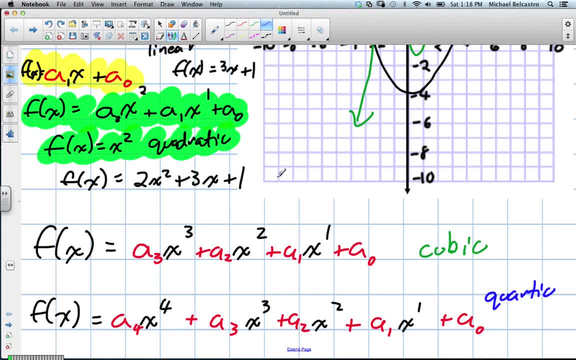 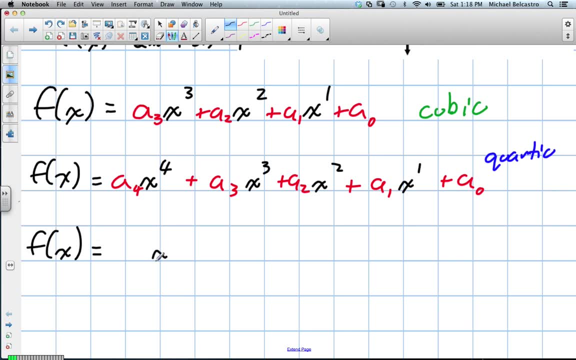 So the last one, I don't even remember what the fifth one's called Quintic function. Okay, Okay, Okay, Okay. Okay, We have names for all of these, but the idea is, you just want to get a feel for what these are going to be like. 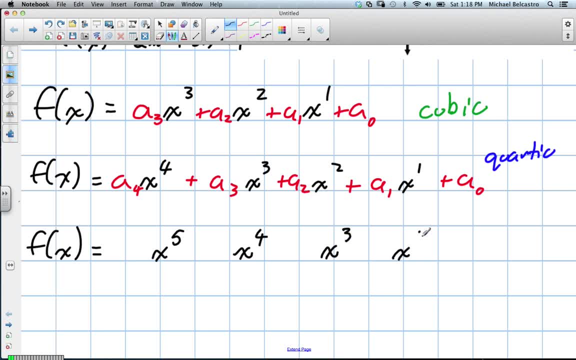 Okay, So all we're doing is adding another variable to each of the equations here. Oops, That should be the power of 1. And there's going to be 5.. They could be the same constants, but in this case there's five different constants or coefficients. 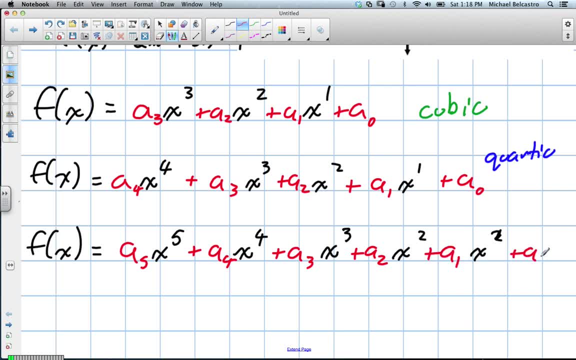 Sorry, not constants. And then there's one constant at the end, which is our a naught Could be some term. Usually that's our y intercept. So if this is a quintic function, have I done right in it? No, I don't think so. 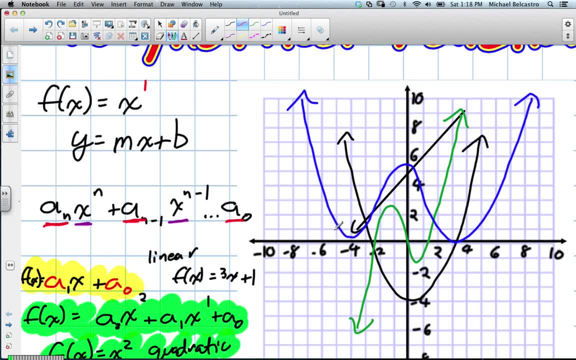 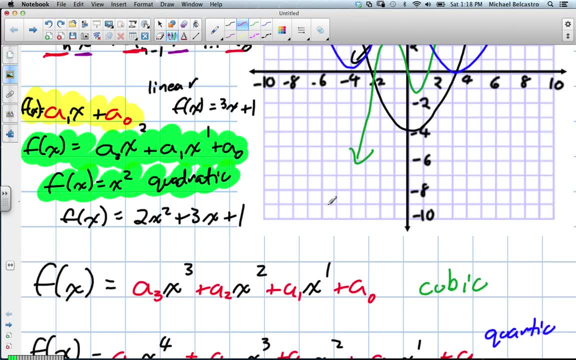 Quintic function okay, So this one's going to have five turns to it, Or sorry, four turns, because we take five and we subtract by one. So I'll try to do this one below, so it's a little easier to view versus the other one. 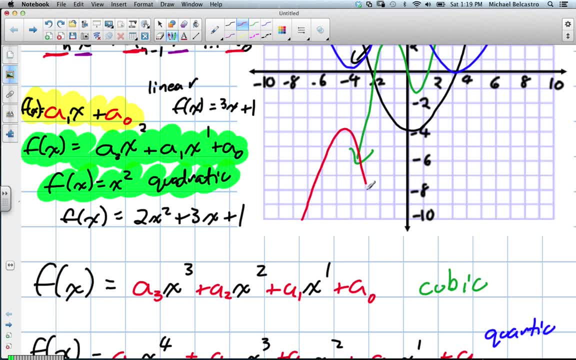 So say, we're going from left to right, We go up, we change directions once, twice, three times, four times, And that's that function there, okay. So the amount of changes in direction of the function is related to essentially what the highest power of a variable is. 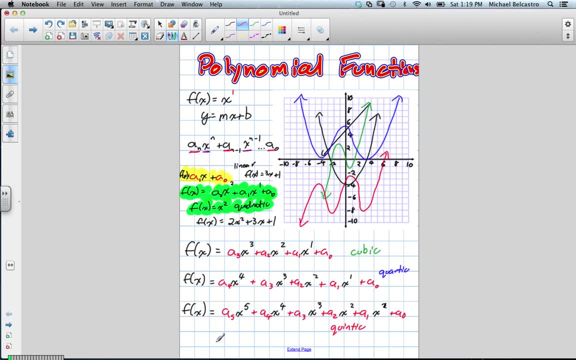 That's what happens to all of these. So what we're going to do is we're going to bring these up and just kind of play around with them a little. We'll look at the originals of each, And what I mean by the originals of each. I've written them all here. 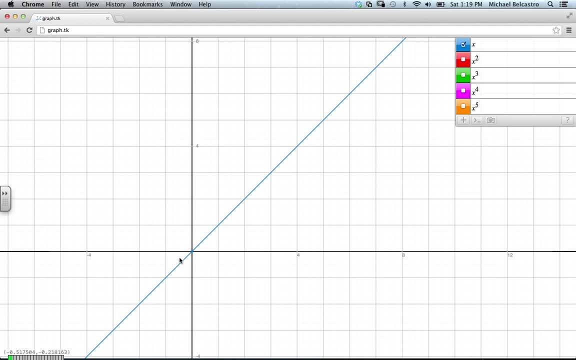 The first one's just a linear function. This is x to the power of one. If you notice, it's a straight line going through the origin. All of these will go through the origin. okay, because I haven't added anything else to them. 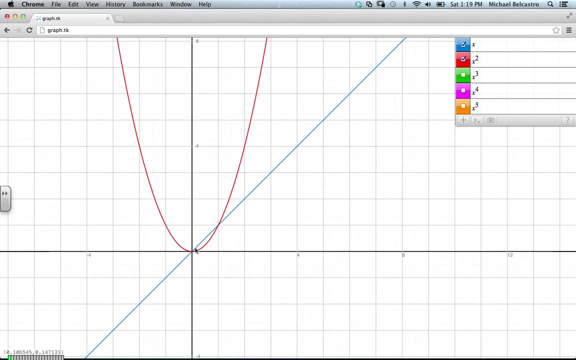 We're used to seeing a quadratic function. It has one turn. okay, Now I'm going to take away the quadratic and the linear just for a second And we're going to look at a cubic function. Now this kind of looks like it's only turned once but it technically is turned twice. 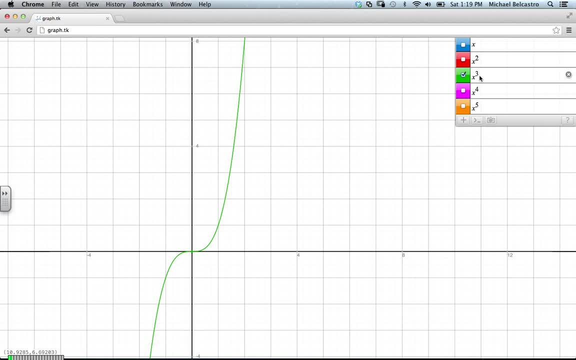 It's very hard to tell. So what we're going to do is we're just going to add a little to this function here. Let's see if we can't Plus x squared, There you go. So I've just kind of added a little to this function. 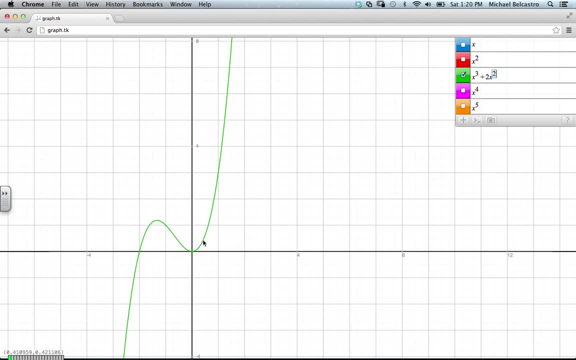 And if you notice it turns once and then twice. okay, That's what's important about this here. The original one did technically do that, but it was much harder to see. okay, So as we play with these functions, we're going to see that they change different direction. 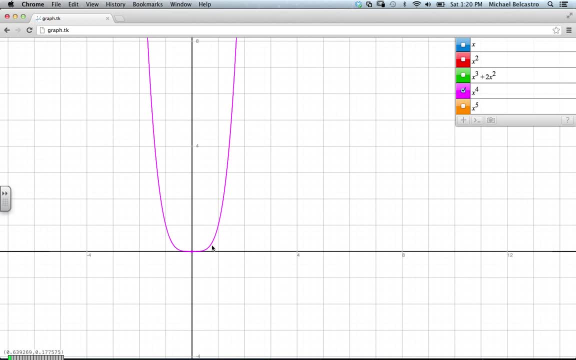 The fourth one here. turn it on almost looks like a parabola. It looks like it's again only turning once, but it's actually turning three times, And what we're going to do is we're going to add a little to this function, like we said. 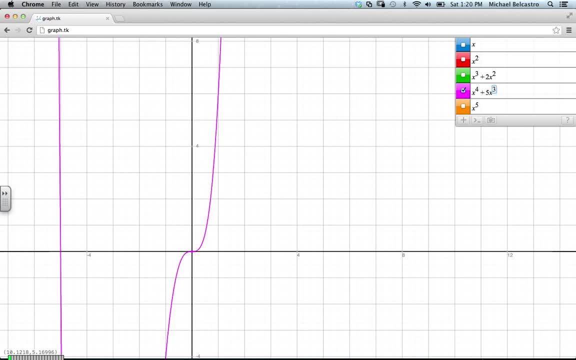 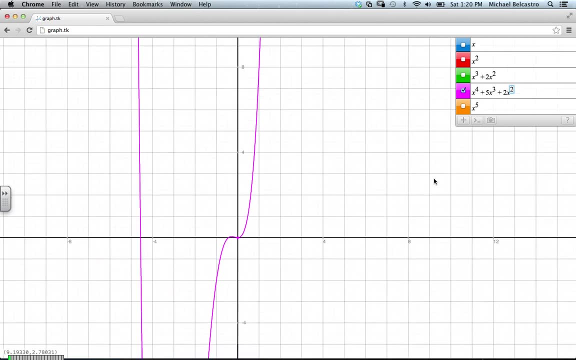 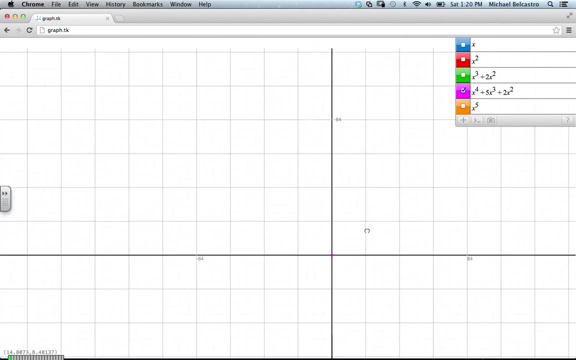 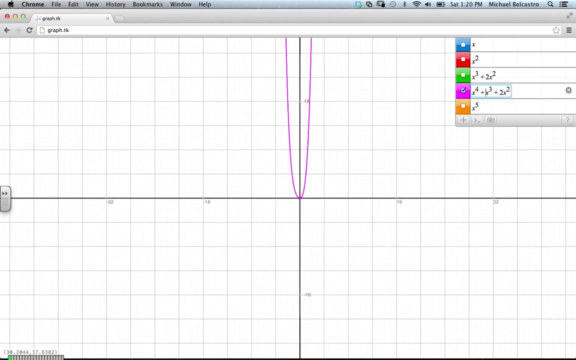 Let's say 5x cubed plus 2x squared. Let's see if that gives us anything. Oh, this one, That's still a little hard to tell. Let's change this number here. Let's admit a bit. Oh, still hard to tell. 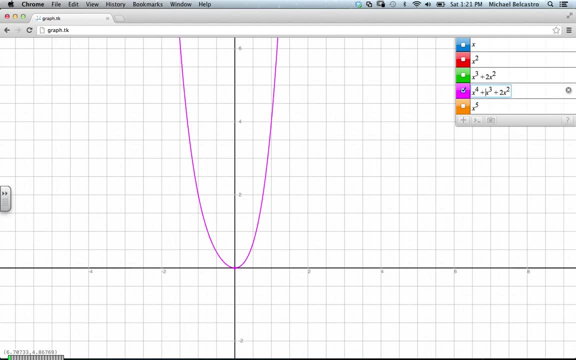 We'll play around with these numbers here. Let's see if we get something that is somewhat. Let's just add. Let's add x. Hmm, Okay, We changed the coefficients to each. We should be getting a four function. What we'll do is: 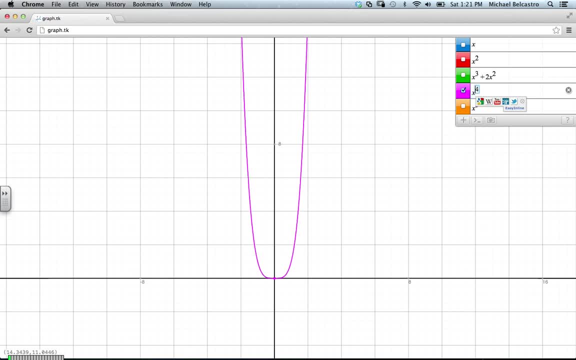 Okay, Take that coefficient away. Let's just see if we can add x. Let's see if we can add x squared. We can zoom in. We can kind of see this. It should have chosen a nicer function that has a more pronounced turning. 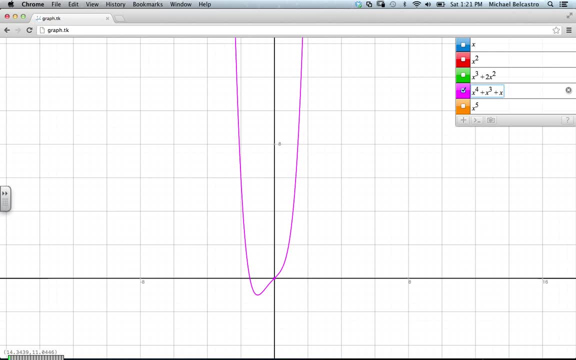 But if you notice this function from left to right is going down, turning once, Then it technically turns twice and then a third time. It comes back up here. What would be a good function? Let's see if they have one for us. 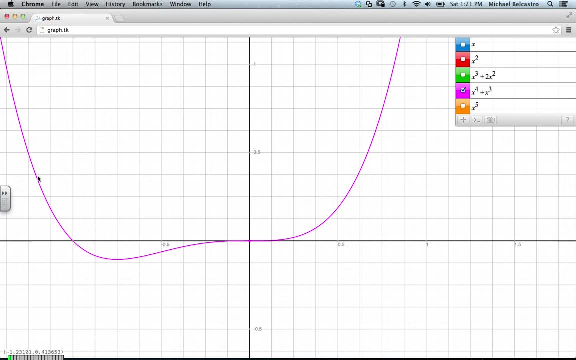 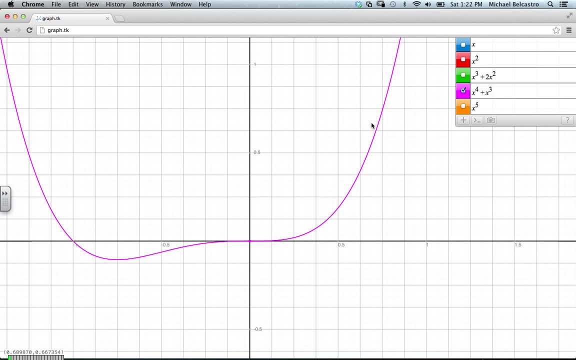 Not this one, Not this one, Not this one. Really We'll get into after, I guess. Okay, So that's our cortic function. This would be This one here. If you notice, it changes three times One. 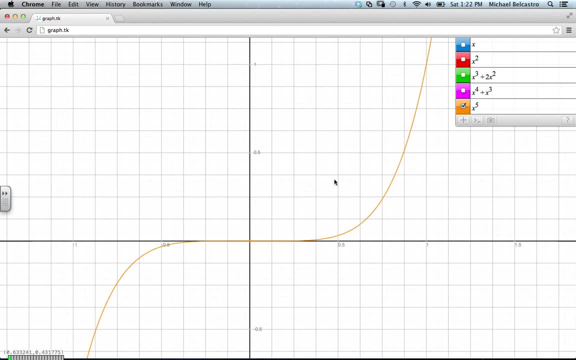 Two And then three times It changes direction. So that's the idea of it. And then the same thing is said for here. Now, this one almost looks like a cubic function. Again, It looks like it's only changing once. 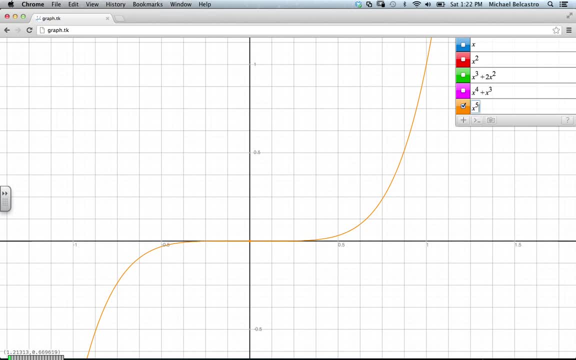 But it's actually changing direction when we get into it four different times here. Let's play with some numbers. Let's hope that x to the power of four- oops, no, x to the power of 4 doesn't do much, minus 5x to the power of 3. 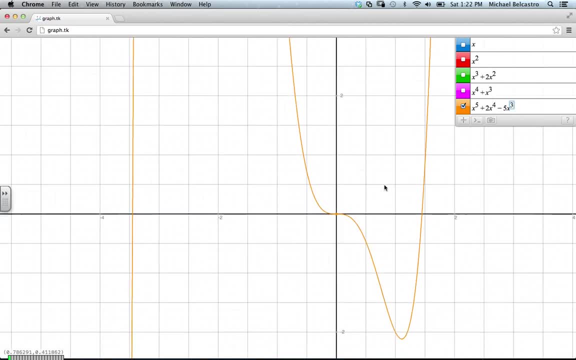 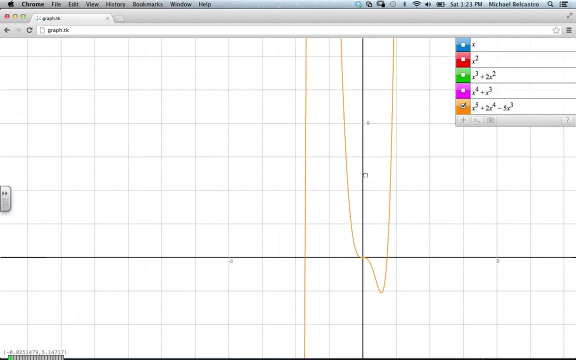 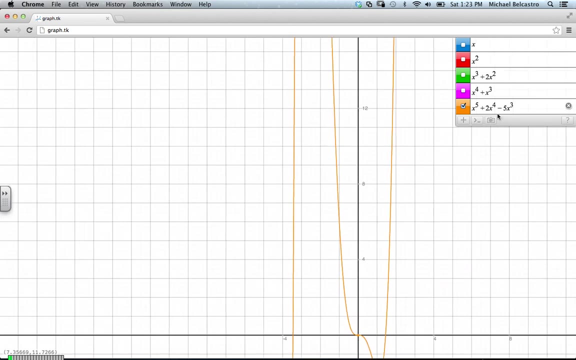 let's see if that does anything for us. there we go. we just need a couple negatives. oh, this one really took off. change that value to 1. there you go: 1, 2, no, it only looks like 2 still. 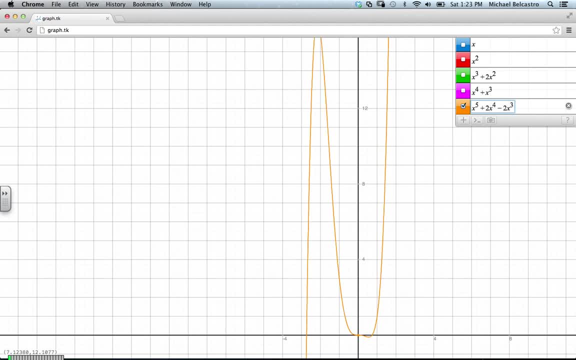 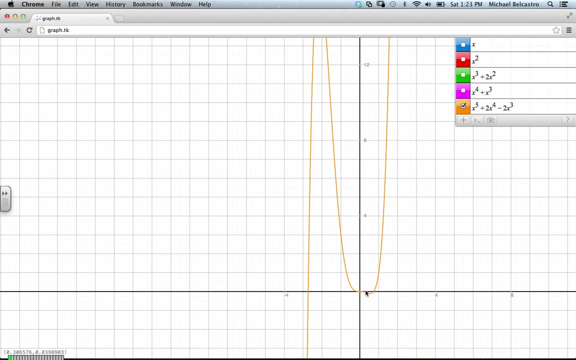 there you go a little bit better. so if you notice, when we go left to right, this goes up, changes direction, once comes down, changes direction twice, 3 times, 4 times. though they're not very pronounced, we'll try to zoom in a little. 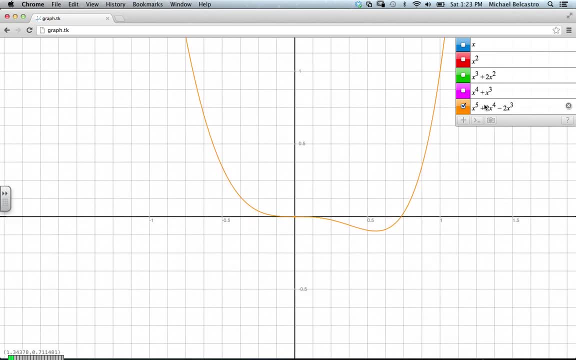 these are changes in direction. so essentially the idea is: for every variable or exponent we add the graph in general just changes a direction another time. so that's what we've got to get used to looking at.